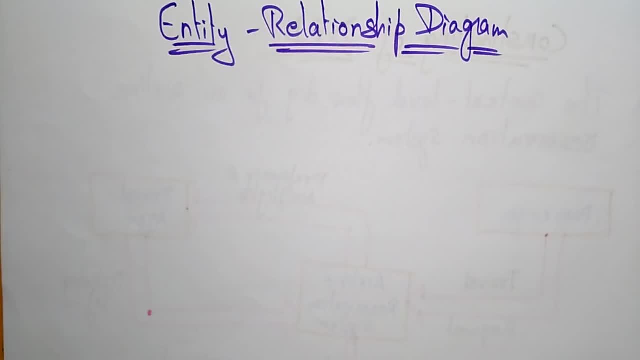 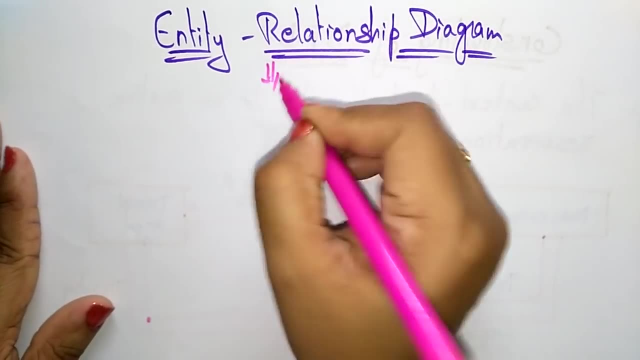 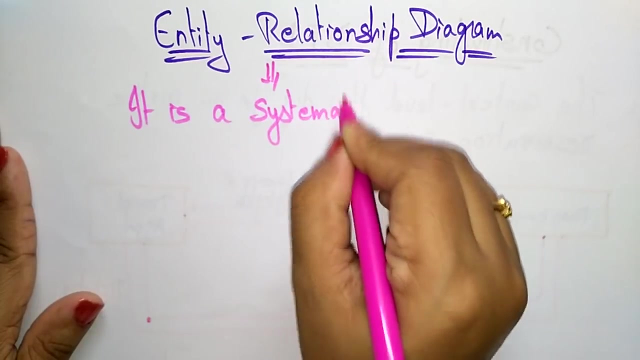 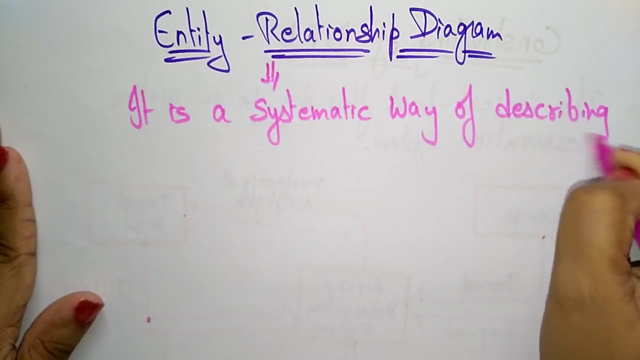 Hi students, coming to the next topic, that is, the Entity Relationship Diagram. So what is this Entity Relationship Diagram? We call it as ER Diagrams. This ER Diagrams, it is a systematic way. It is a systematic way of describing and defining. 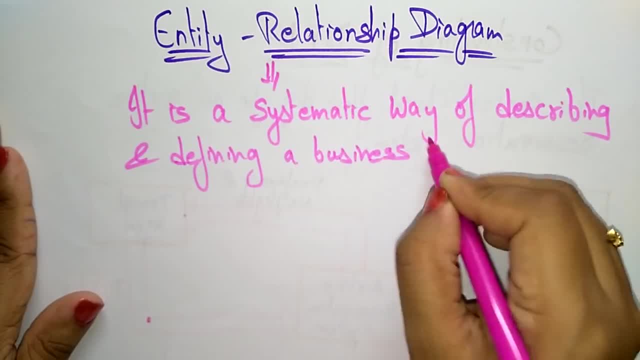 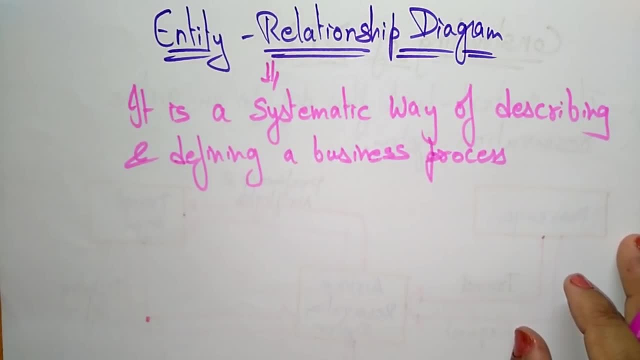 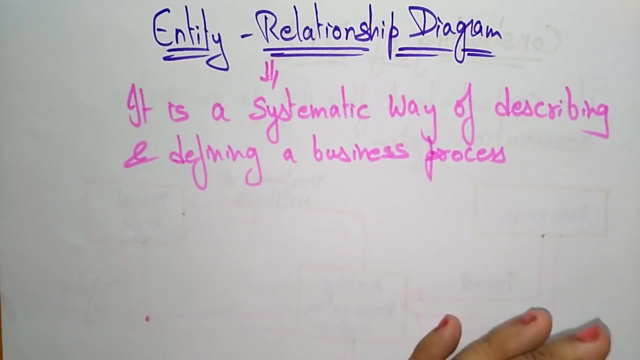 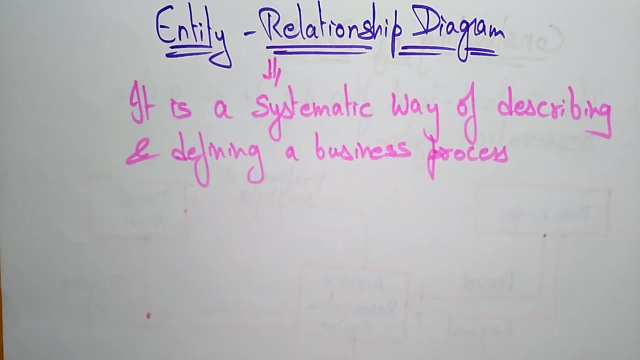 a business process. So to describe and design a business process we need one systematic way. That systematic way is the Entity Relationship Diagram. So the process is modeled as component entities that are linked with each other- So whatever that is there in this with each other by relationships that express the dependency and requirements between them. So different entities will be there means different persons will be there. 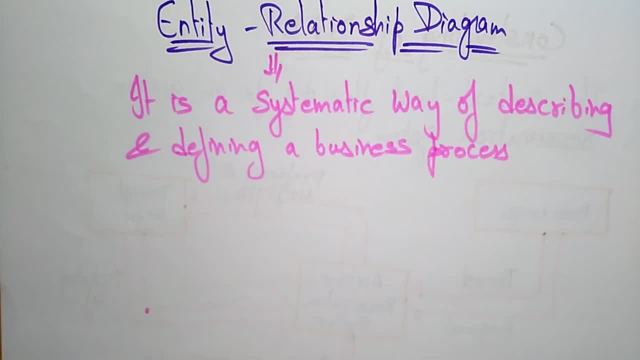 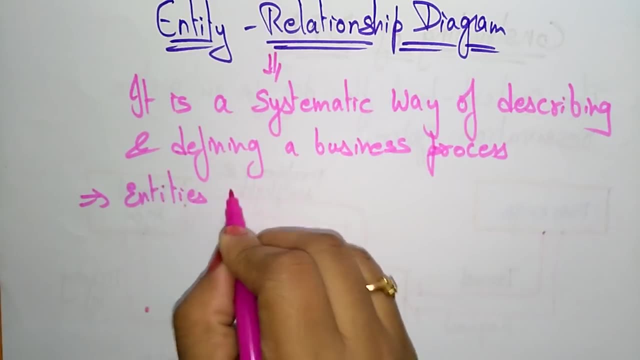 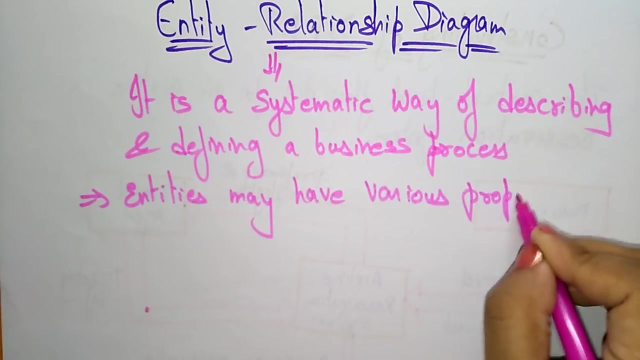 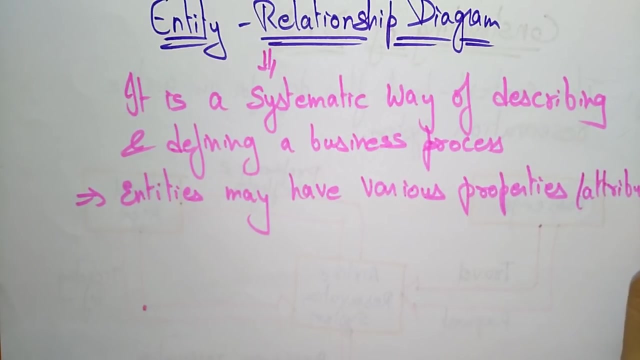 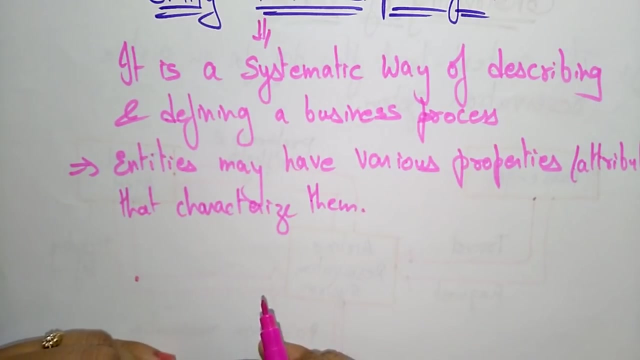 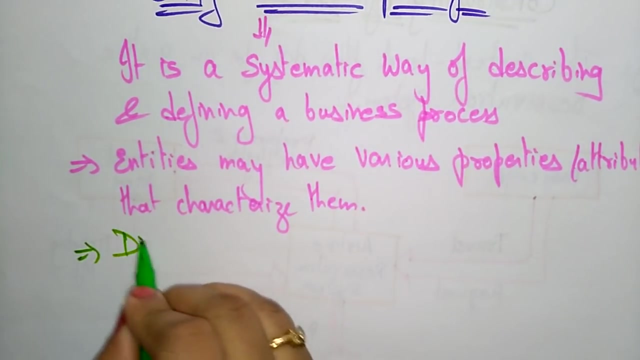 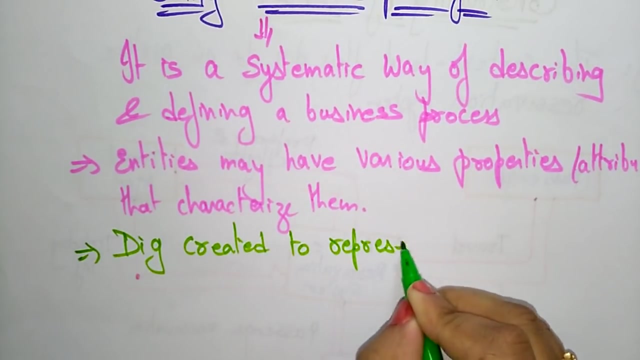 So a communication between those persons can be represented by using Entity Relationship Diagram. Here the entities- entities may have various properties that you call it as attributes. Each entities have various properties, attributes that characterize them, And this diagram is going to create a diagram created to represent these entities, attributes and relationships. Let me write that: A diagram created to represent these entities. So, whatever the entities that we are using, these entities- 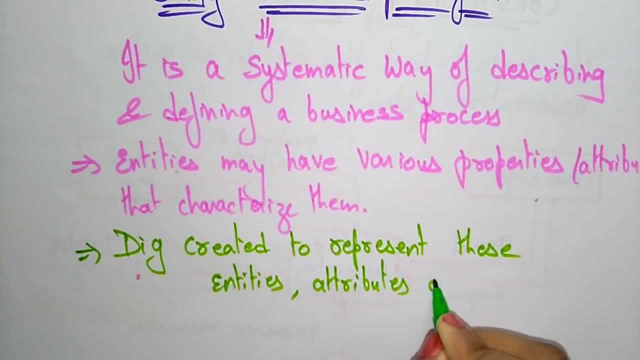 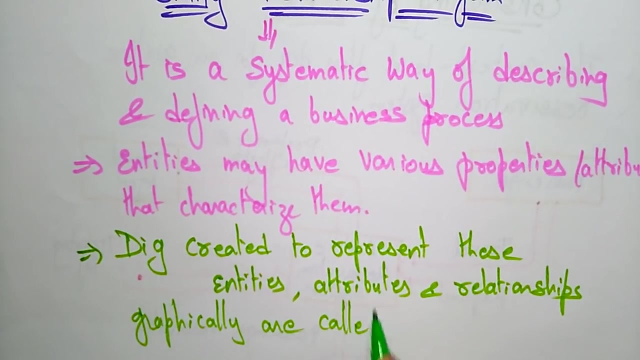 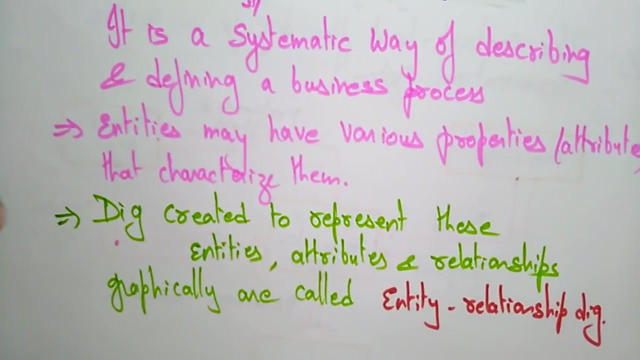 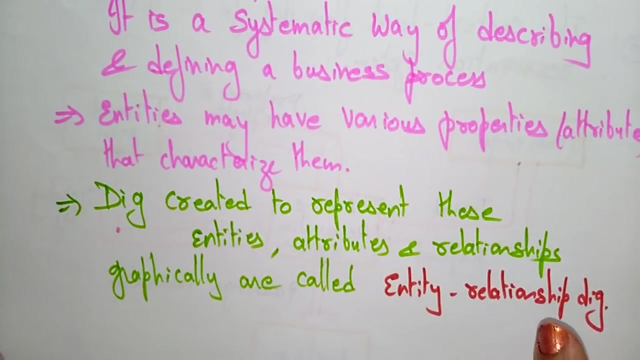 These attributes and relationships between those entities and relationships graphically or called graphically, or called Entity Relationship Diagram. Okay, So the Entity Relationship Diagram is nothing, but it is going to represent the entities, attributes and relationships graphically or called Entity Relationship Diagram. 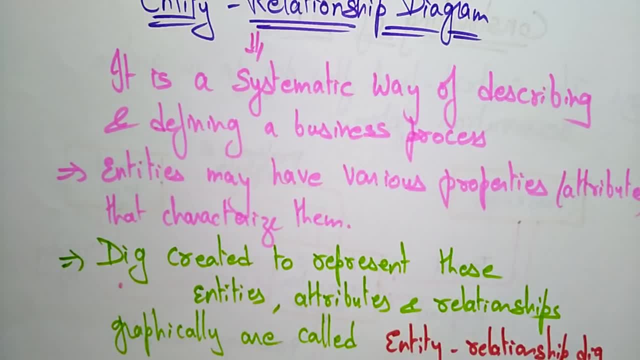 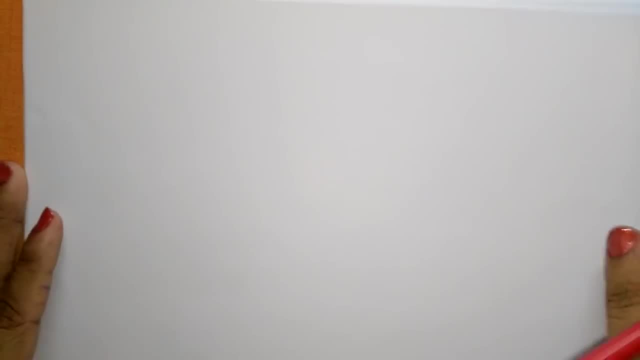 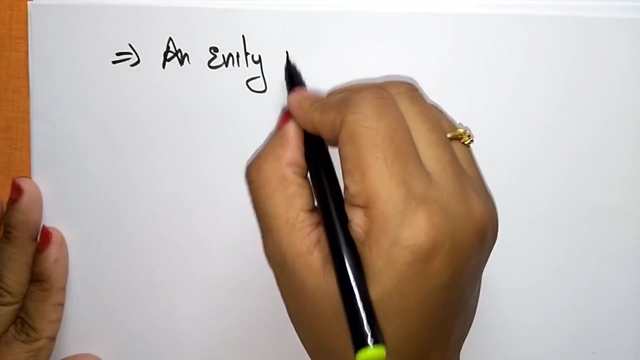 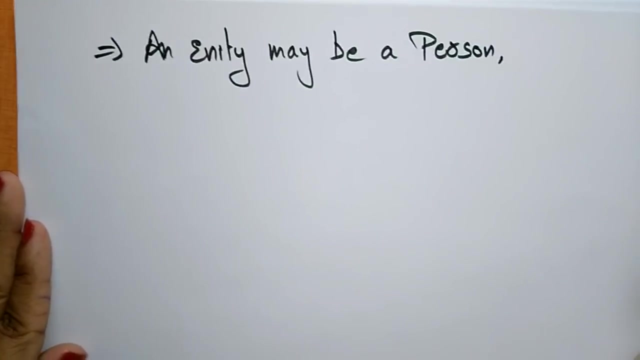 So the main use of this Entity Relationship Diagram. it is a systematic way of describing and defining the business process. So what is an entity exactly? Entity is nothing but an entity. Maybe you call it Entity is maybe a person. the entity may be a person, place or thing. 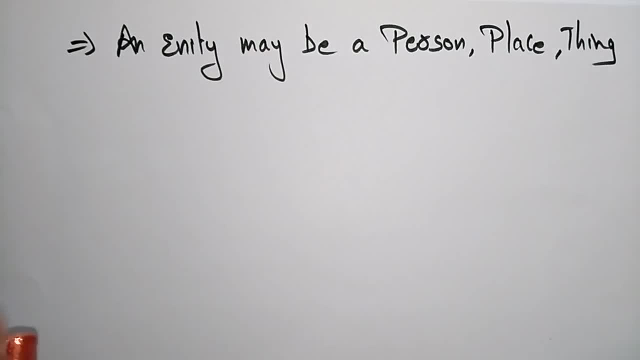 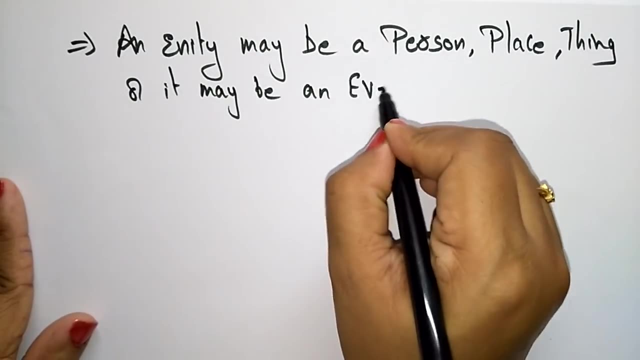 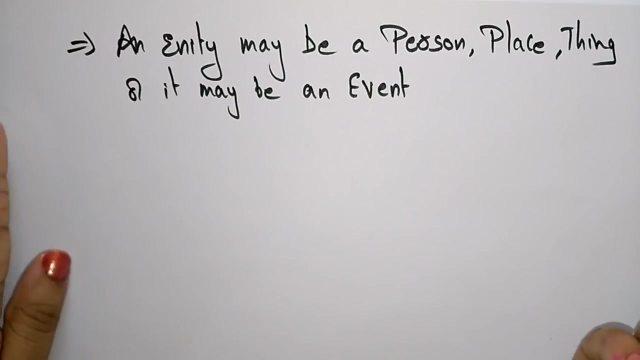 You call that entity. may be a person, place or a thing, or it may be, it may be an event. Not only a single person, single place, single thing, It's just an entity. Sometimes it may be an event Also. 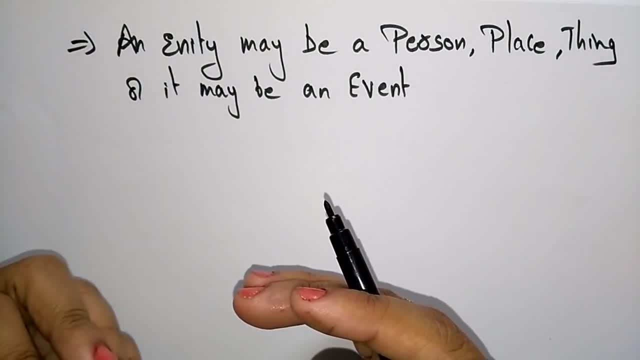 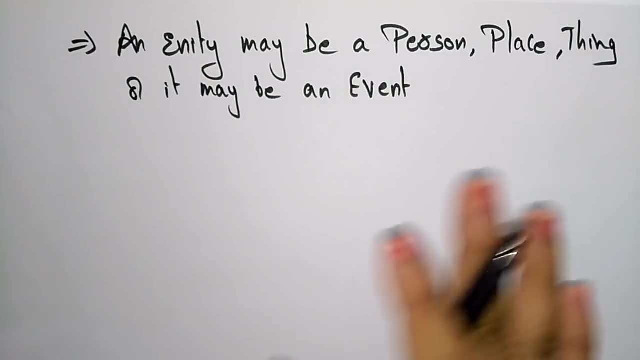 So event like the month and the sales period and the machine breakdown means some action that has performed that as an entity, A relationship is associated that describes the interaction among entities. So here a relationship will be used to associate that describes interaction among those entities. 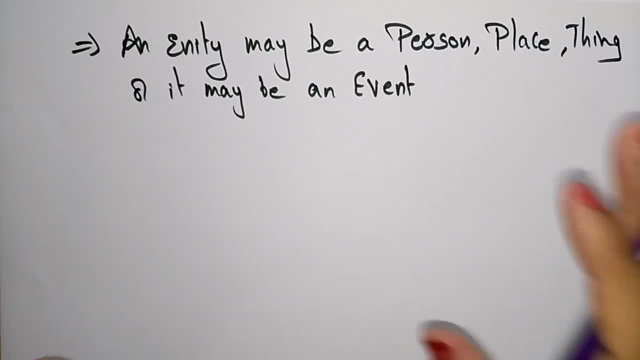 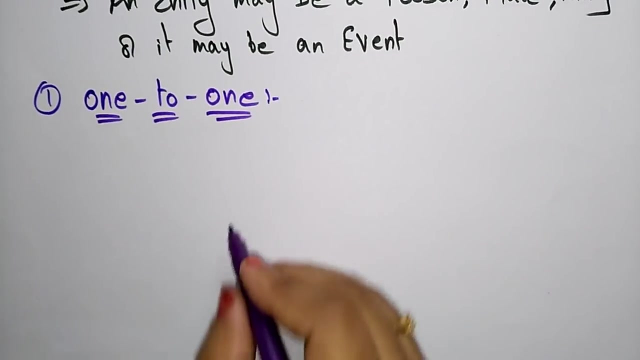 Now let me explain the different entity relationship diagrams. So first one is one to one entity Entity relationship diagram. One to one entity relationship diagram. So let us take here An employee was there Employee And here the phone extension will be there. 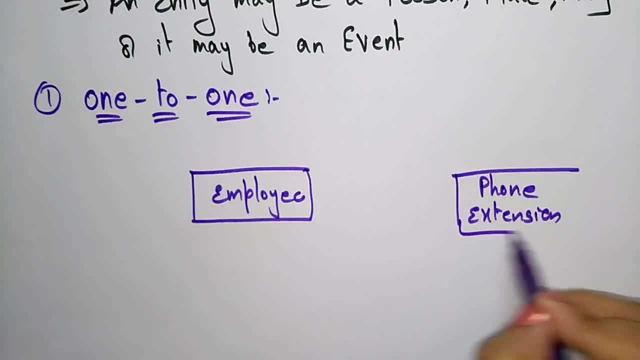 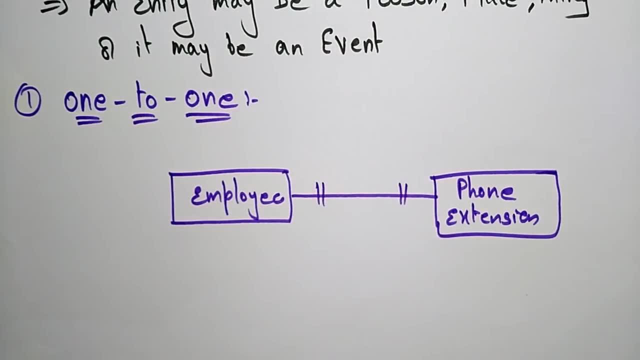 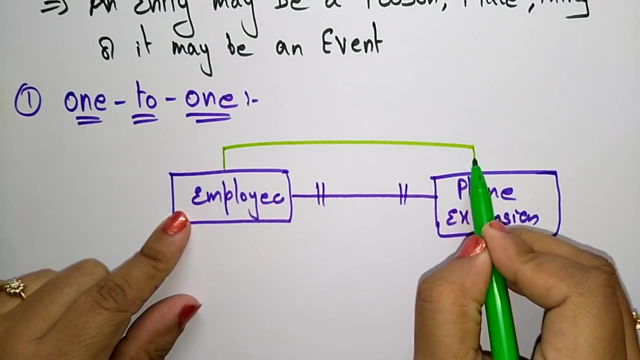 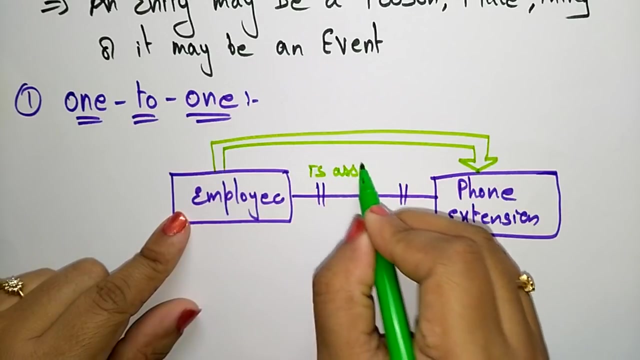 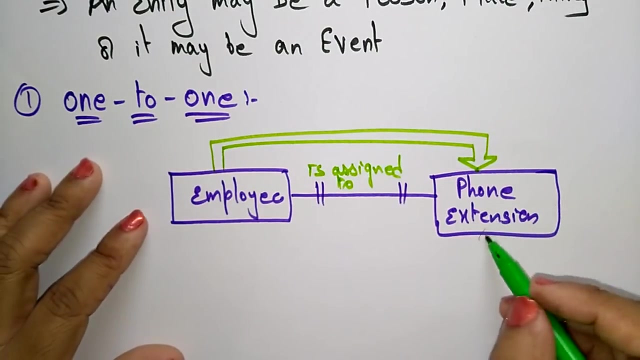 Phone Extension: Okay, Okay, Okay Is, And it. so here the employee is assigned to an extension that employee is assigned to Next exit extension is sign To Foreign extension and the foreign extension The The foreign extension. 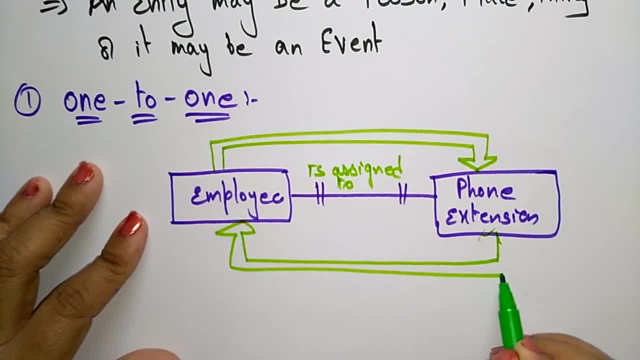 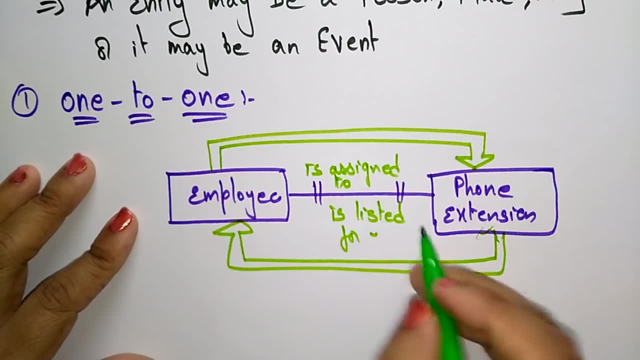 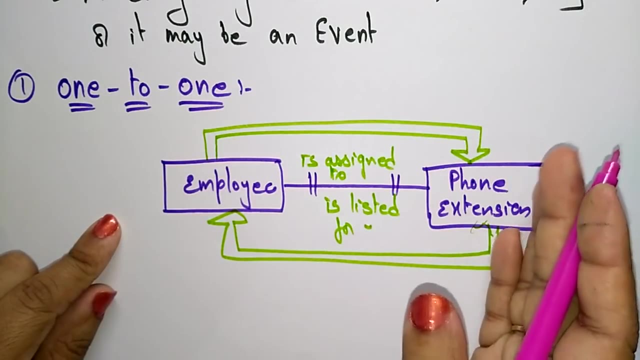 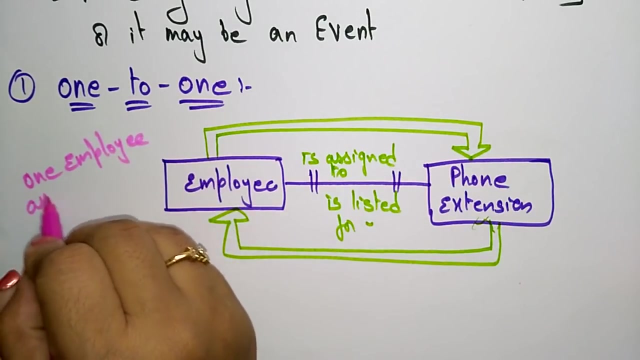 On the, The, The ared Next phone extension is listed for employee. is listed for employee. so what is saying that? so here one employee is assigned to only one phone extension. one employee assigned to one phone extension because he can only talk once means if we are talking on one phone, we are not supposed. 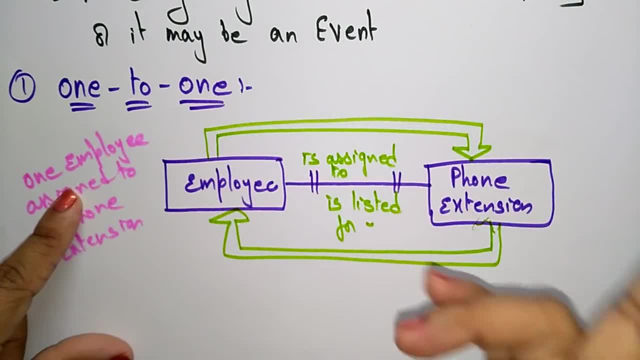 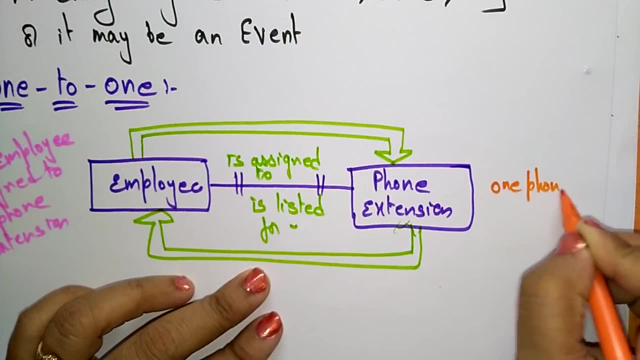 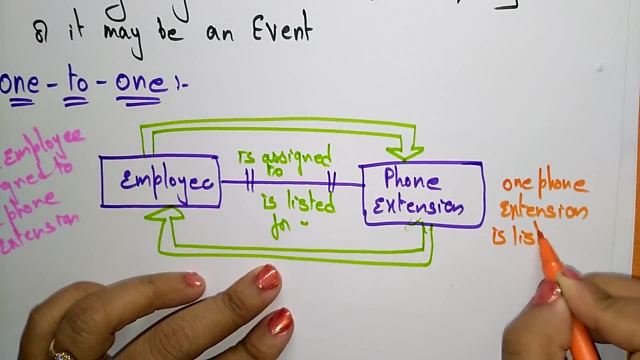 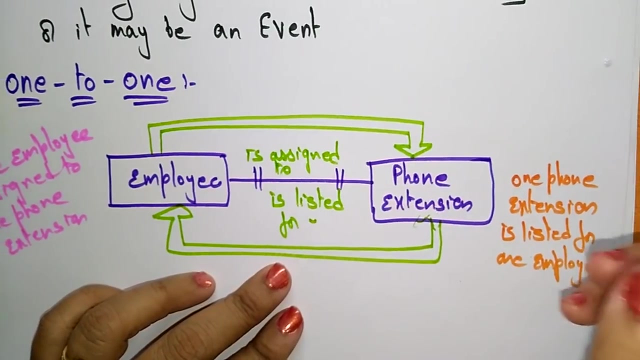 to take another call. so one employee is assigned to one phone extension, whereas here one phone extension, one phone extension- is listed for one employee, so only one phone extension is in the list. start with that number. one phone extension. phone extension is listed for only one employee and one employee is assigned to only one phone. 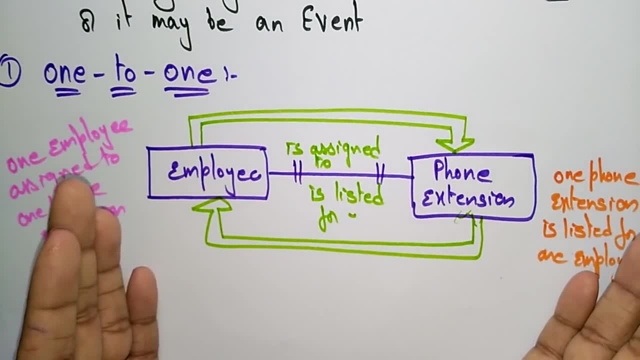 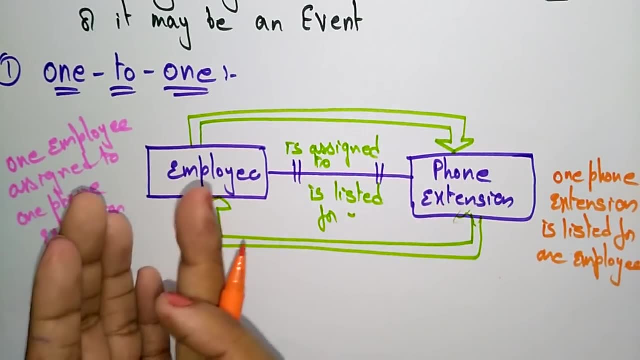 extension. So this explains the one-to-one relationship, one-to-one entity relationship diagram. So this is an entity. employee is an entity, phone extension is an entity. So here this explains the entity relationship diagram. that is a one-to-one. Now let us see the second. 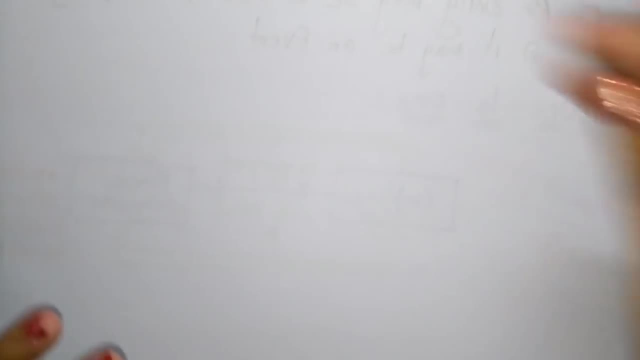 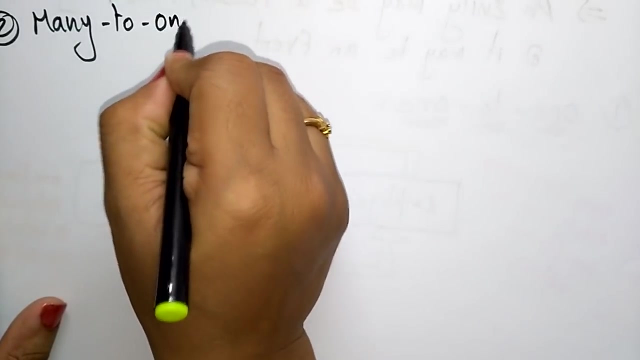 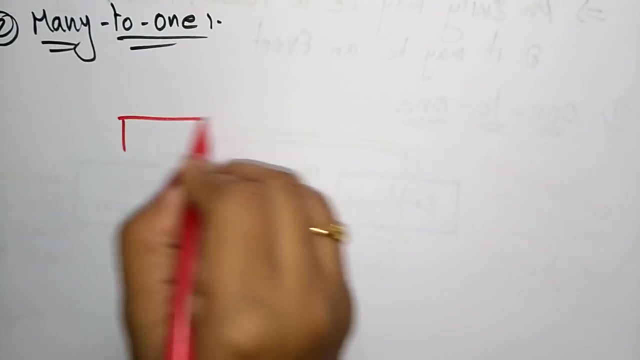 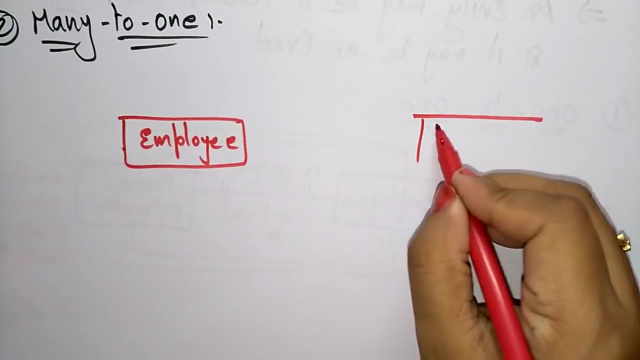 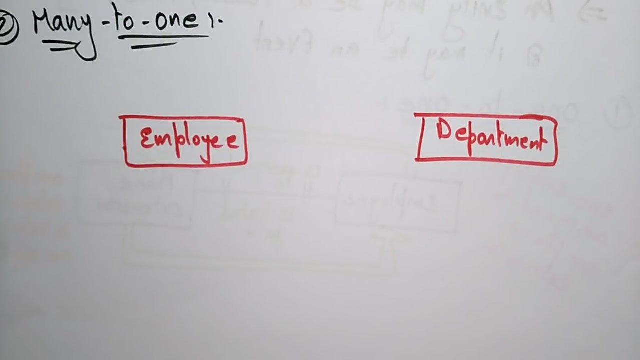 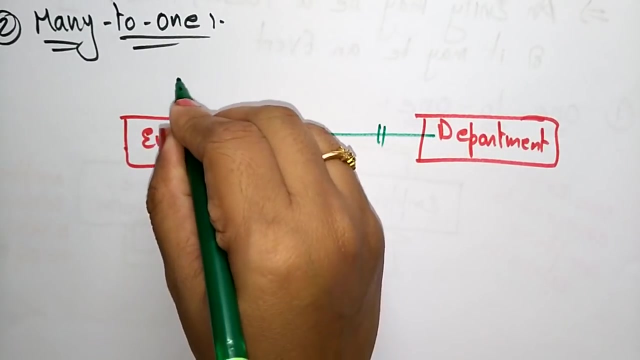 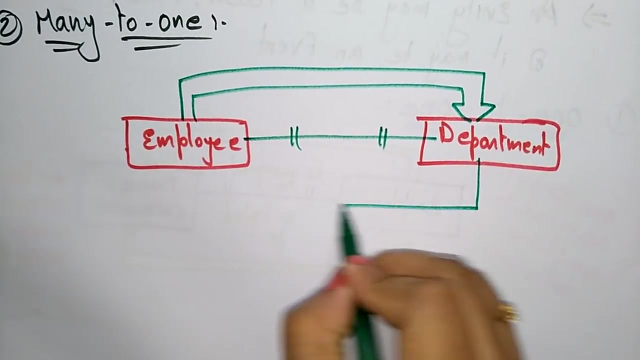 many-to-one. The second one is many-to-one entity relationship diagram. So here I am taking employee and department, Employee and department as two entities. So here a communication between these, and this department is going to communicate with the employee. 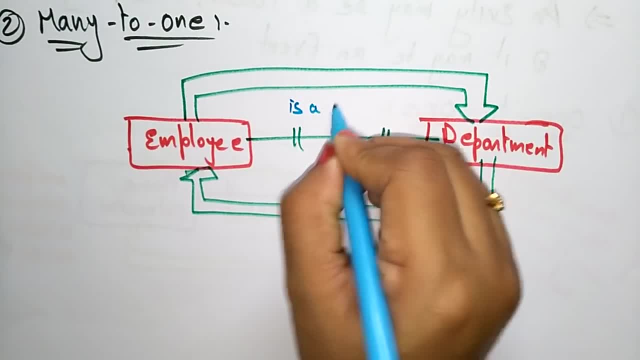 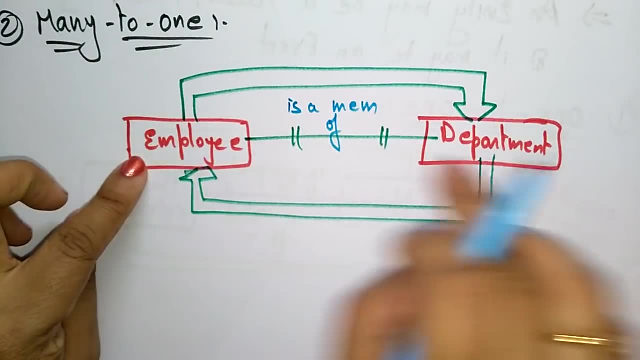 So here, employee is a member of a department Is a member of a department. Any department is a member, Any department is a member, Any department is a member department. there are so many employees, so many to one. many employees are working in a single. 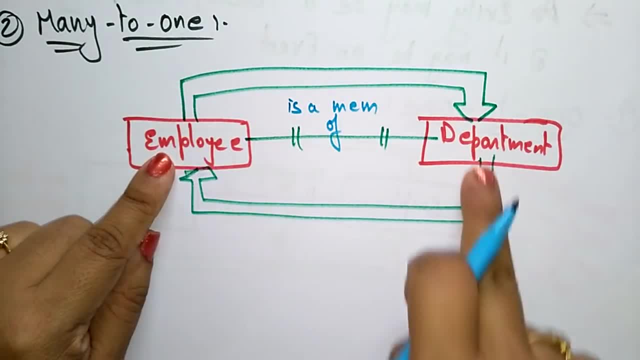 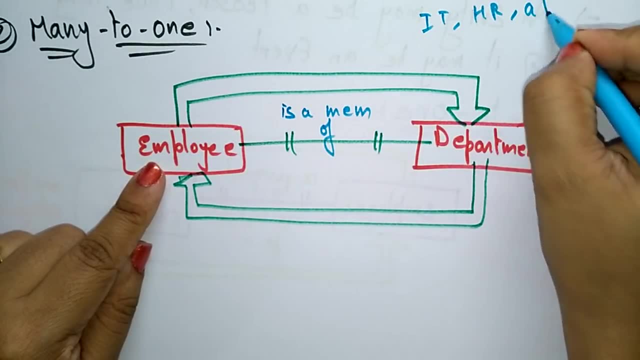 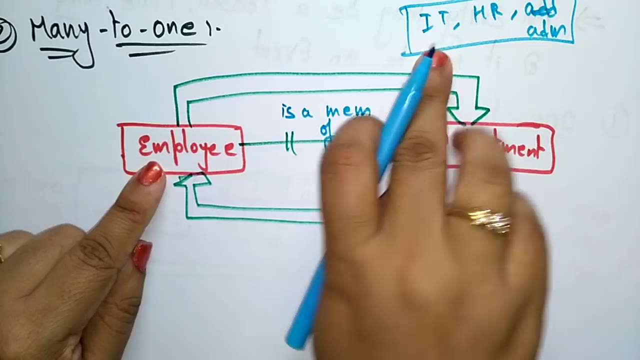 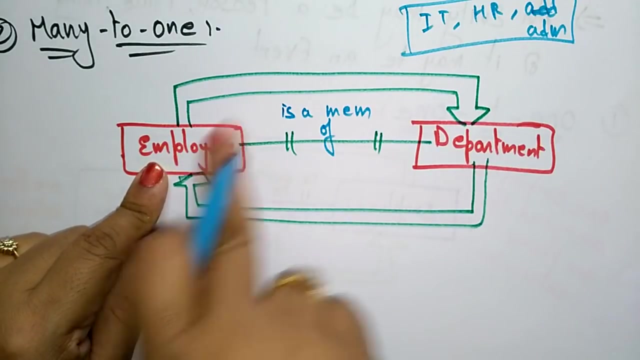 department many to one. many employees or work in a single department. suppose different sectors are their IT sector, HR sector, so different sector, administrative sector, so different sectors will be there in any organization. so each department is having set of employees. so a number of employees are working in a single department. so employee is a member of a department, whereas department 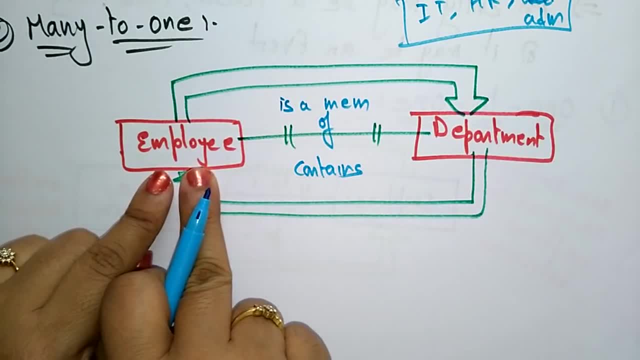 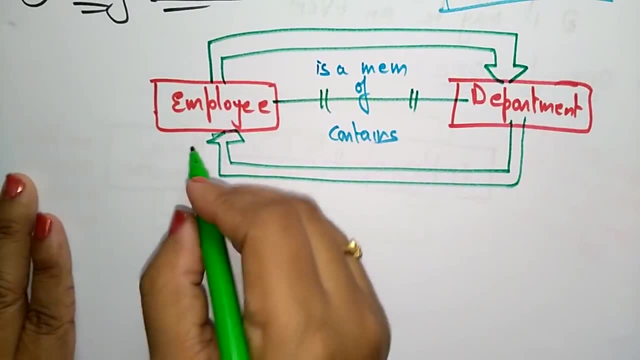 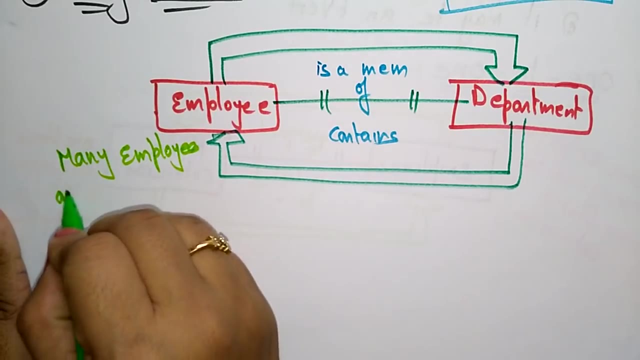 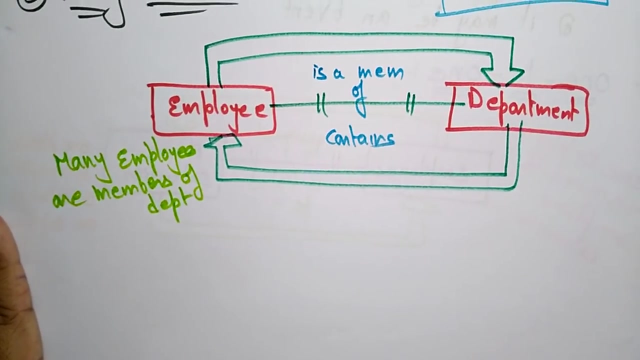 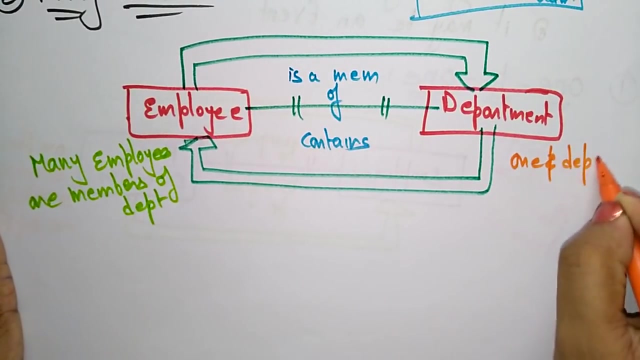 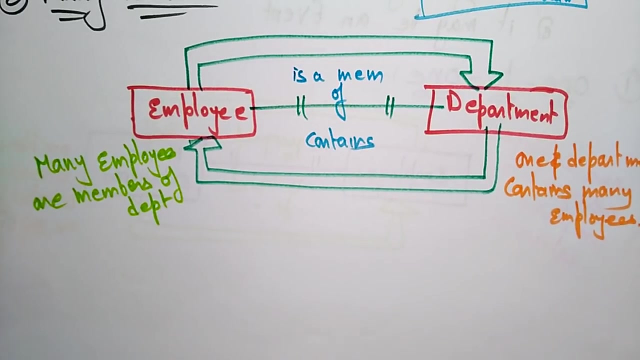 contains employees. department contains employees, employees, a member of department. so here it's saying that employee, many employees or member of the part, members of the department, many employees or members of department. and here one department, one department, contains many employees. so this shows the many to one relationship. one, uh, one department contains 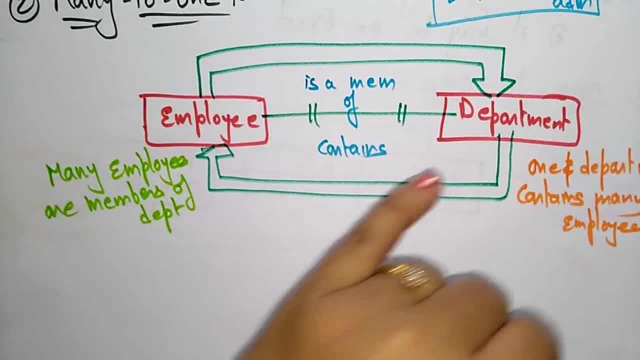 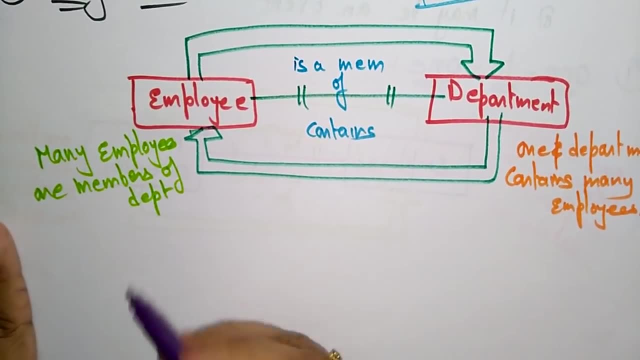 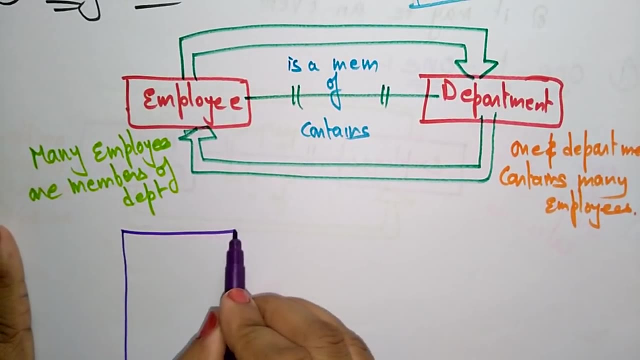 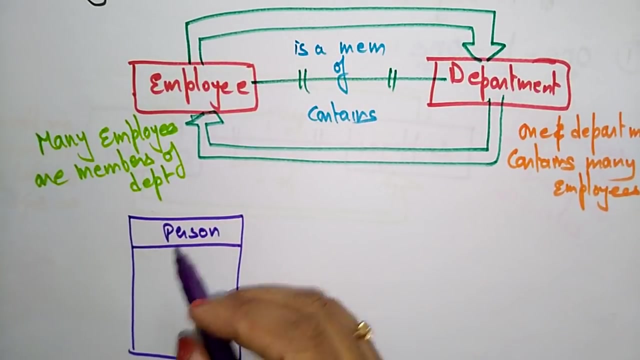 many employees. so many employees can work in one department, so this can be also represented by using the class diagrams. let me show you that another way of representing this entity relationship diagram is like this: a person will be there, so this is another. another example: person will be represented with 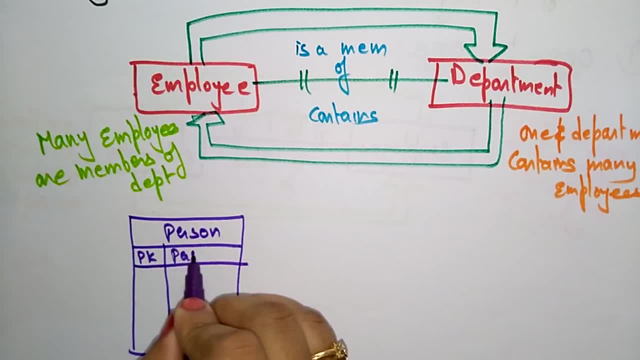 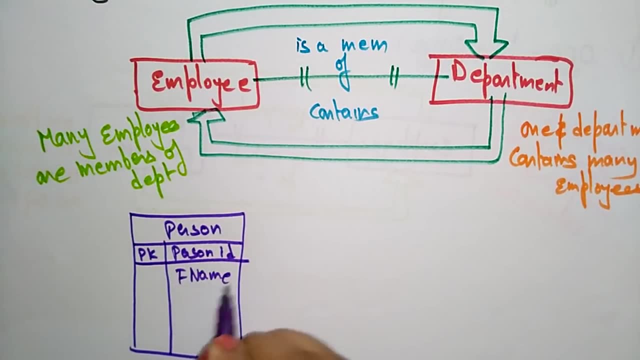 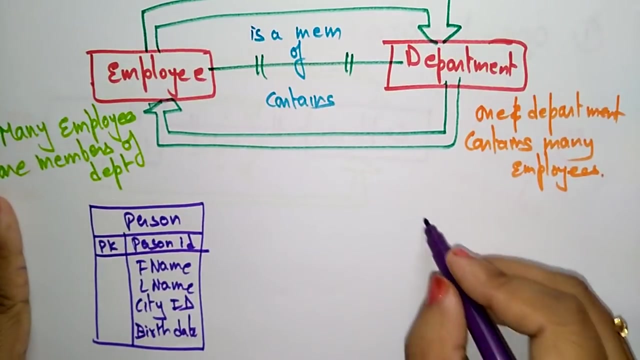 it's a primary key. a single person with person id id is a primary key here: person id, first name, last name. so these are the details of the person: single person, city id and birth date. so these are the details of any person. so a single person. and here you are having it: another class, so that is a city. 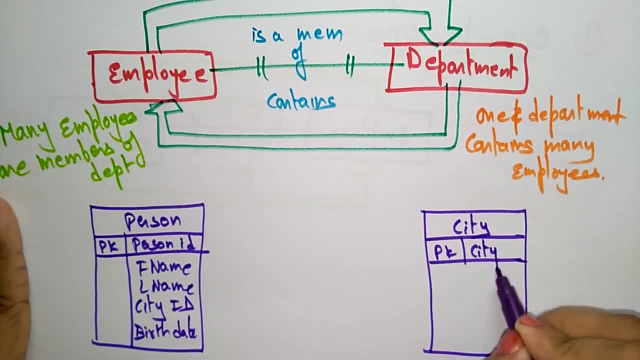 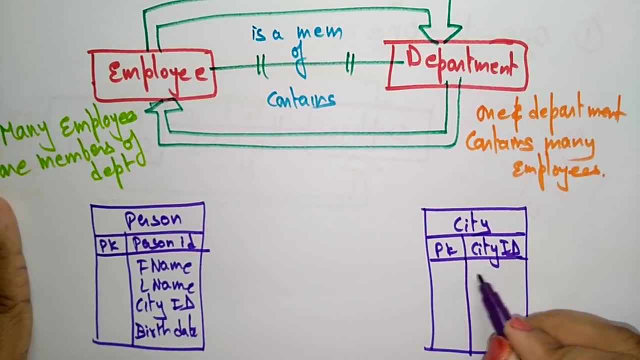 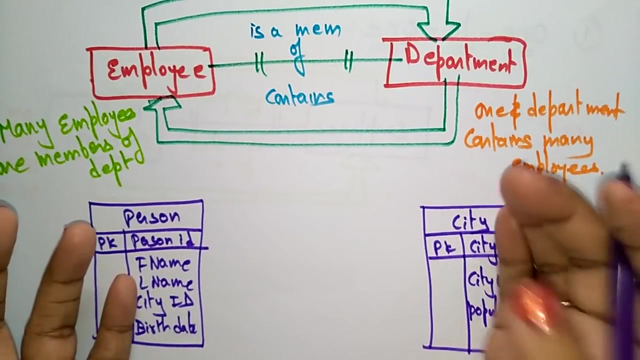 primary key was the city id, because it is unique city id and here i am writing city name and total number of population. so this is a single, a person's, a group of persons and their details, and a city. in a city there are many persons can leave, many people can live in a